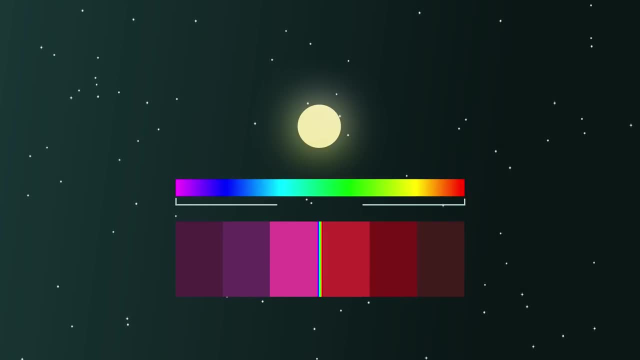 we get from the Sun. You probably know something about the electromagnetic spectrum: rays of energy that travel at the speed of light. Here is the full spectrum starting with the low-energy least harmful radio waves. Here is the full spectrum starting with the low-energy least harmful radio waves. 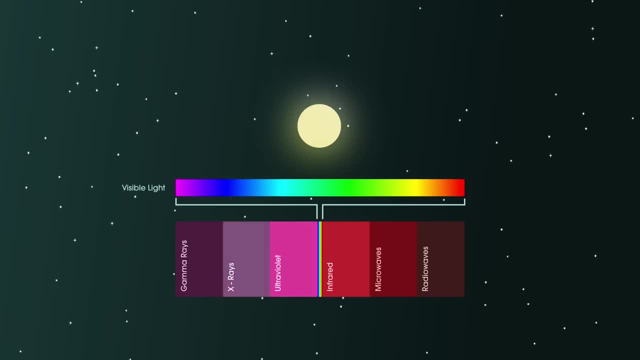 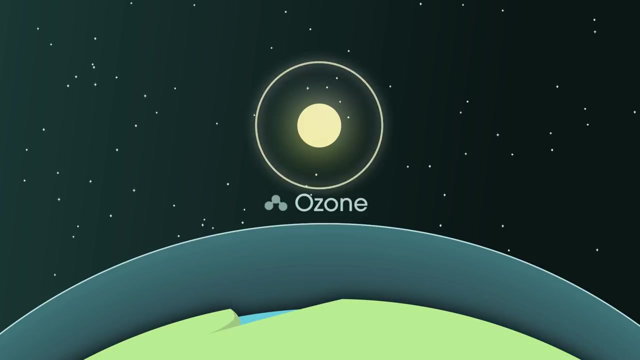 And finally the more harmful rays: ultraviolet x-rays and gamma rays. Most of the energy we get from the Sun comes to us as visible light. Most of the small amount of ultraviolet is trapped in the upper atmosphere by ozone, and there's a linked video for you to see on that, Although enough gets. 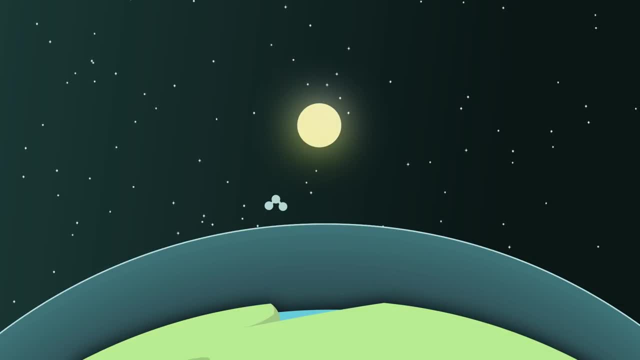 through to damage our skin if we stand too long in the Sun And we only get a little of our solar energy from infrared or heat rays. We only get a little of our solar energy from infrared or heat rays And we only get a little of our solar energy from infrared or heat rays And we only get a. 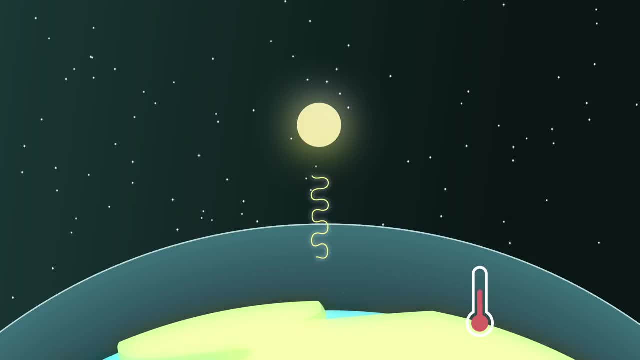 little bit of our solar energy from infrared or heat rays. We only get a little bit of our solar energy from infrared or heat rays, And we only get a little bit of our solar energy from infrared or heat rays. The visible light gets straight through our transparent atmosphere and is partly absorbed by the earth. 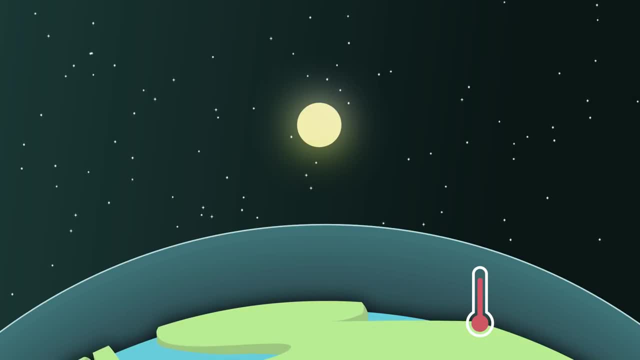 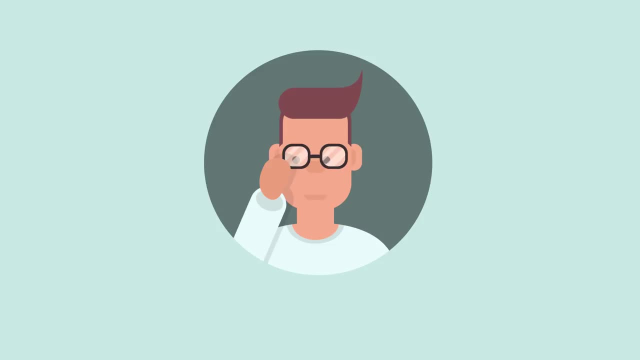 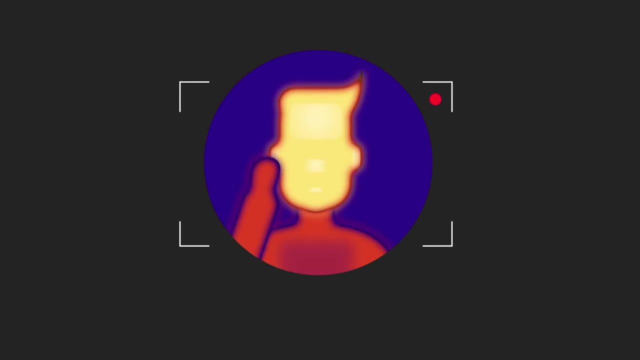 which gets hot. Now, hot things radiate infrared rays. You could try holding your hand very close, but not touching your cheek. can you feel a glow? that's the infrared radiation. infrared cameras can pick up this radiation emitted from warm bodies. now here's the cap. 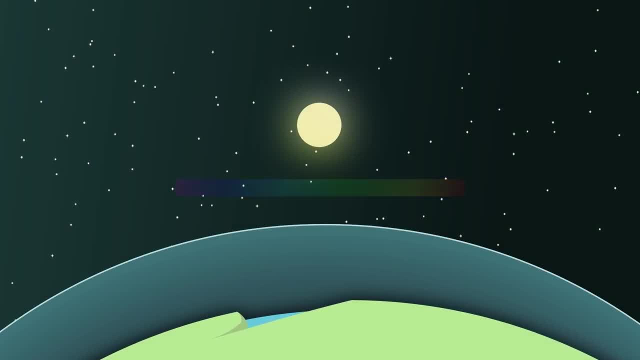 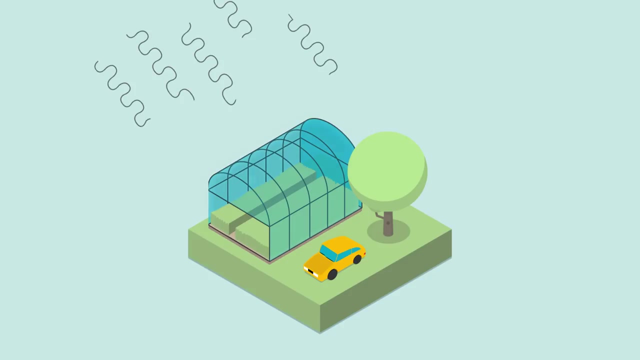 Although visible light got through the atmosphere, the infrared radiation coming from the earth finds it more difficult to get through A greenhouse or even a car left in the Sun works in a similar way. Visible light gets through the glass, heats the soil or the seats which glow, giving off infrared heat radiation. But 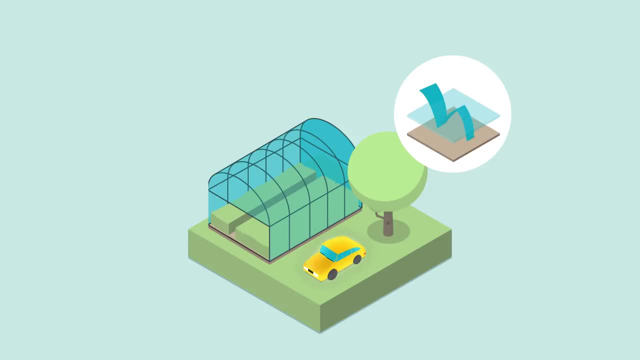 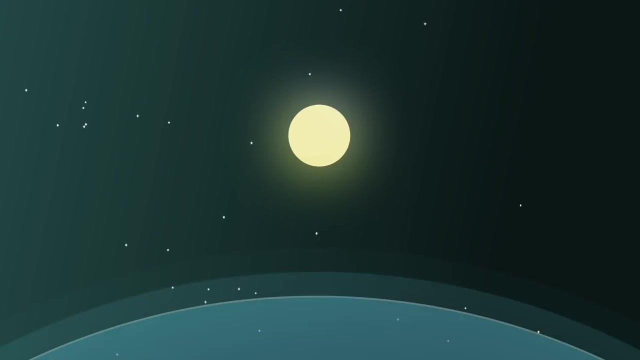 this cannot get through the glass. so the heat builds up inside the greenhouse and the car. So the atmosphere acts a bit like glass, letting visible light through to warm the earth. but some of the heat or infrared radiation now given off gets absorbed by certain gases in the atmosphere, and these are the gases we